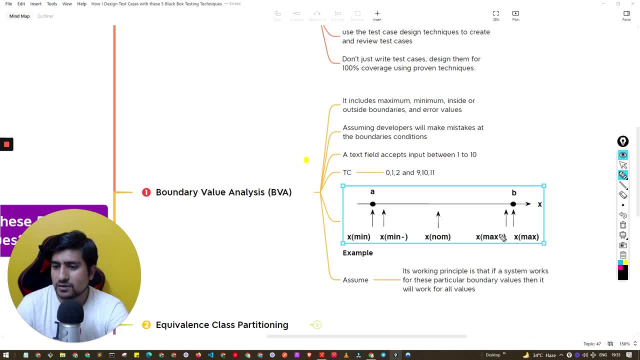 make it small. So here is the first one. Let me get yellow. This is your inputs And this is your boundaries. A and B are your boundaries And so, for example- let's take an example, It's very simple- Suppose there is a text field. This is a text field where you can enter your username. Okay, 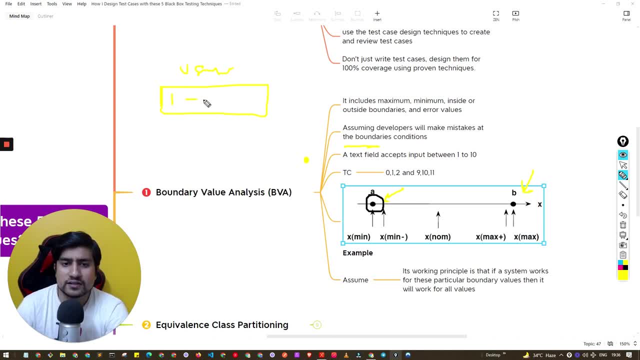 you have seen this many times Now: if you you can enter here, they're saying you can enter the value here. Okay, so what are the cases? What are the different cases? the boundary cases basically says that you can have test zero as your boundary, one as a boundary and two you don't have to test for. 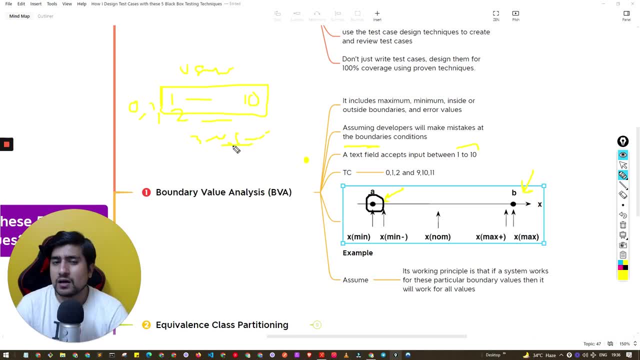 three, four, five, six, seven, because they they will work Mostly. if you see as this basically this technique assumes, it basically assumes, if you see, developer will make mistake at the boundaries. this actually assume the things Okay. so every technique basically assumes something. If you see, 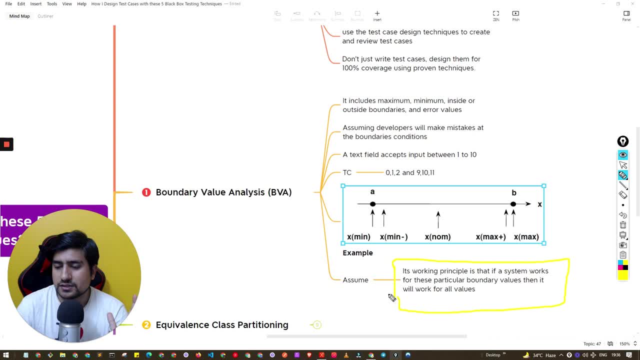 it assumes that the at the boundaries, the there will be errors. okay, because if I, if two is working, fine, then nine will work also fine, because those are very similar and they are not around the boundaries. Okay, so this is actually the boundary value. I hope this is clear. So what? 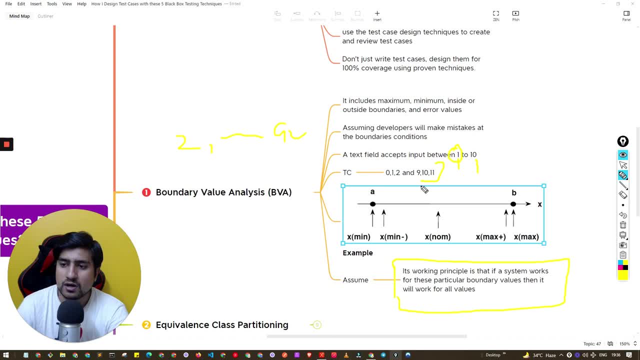 you will do is you will basically create a boundary for this and boundary for this, So zero. So less than this is zero. greater than one is two. So this is your first test cases. So you will test with the zero input. one input and two, So you have three test cases now. 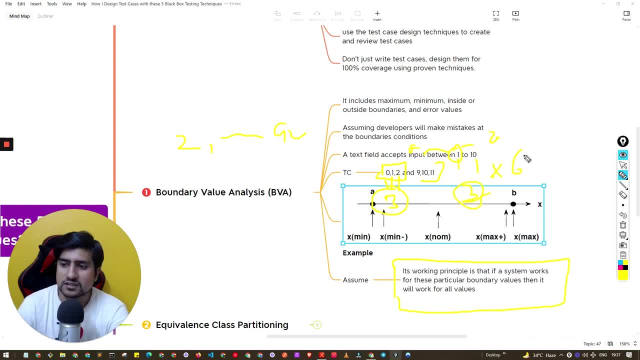 available right and three test cases here. So total number of cases: six. so six test cases, which will basically you are using boundary value analysis and you're done. Okay, let's move on to the equivalence partition. Now This is clear, right? Awesome, Let's quickly go to the equivalence. 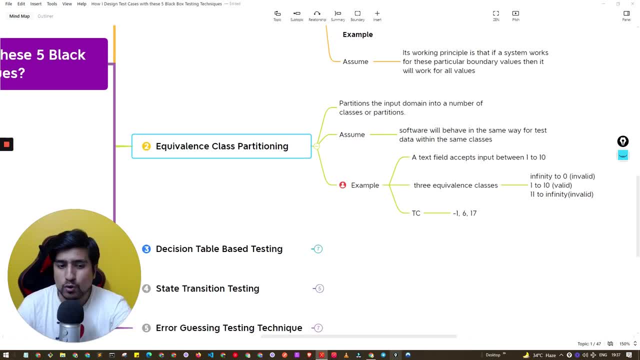 partition, which is very simple In the nature. people make it more complex, I don't know how. So again, same thing. It's basically says: okay, it basically said we are partitioning the input into multiple classes or partitions, So basically we are dividing. suppose similar thing is there. 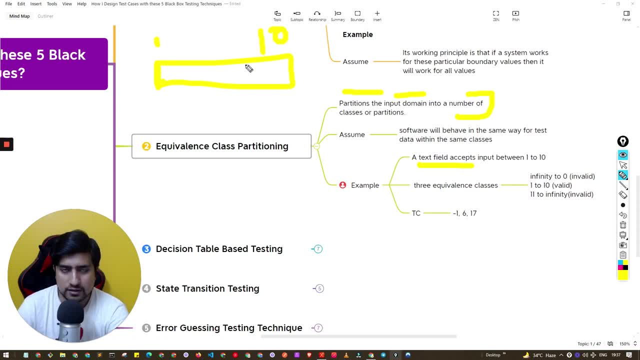 text field that accepts one to zero, one to 10,. right, we are divided into three equivalent part. this is: this is like a negative part, this is positive part and this is negative part. right, Let me use color here. This is your negative part. this is your negative part. 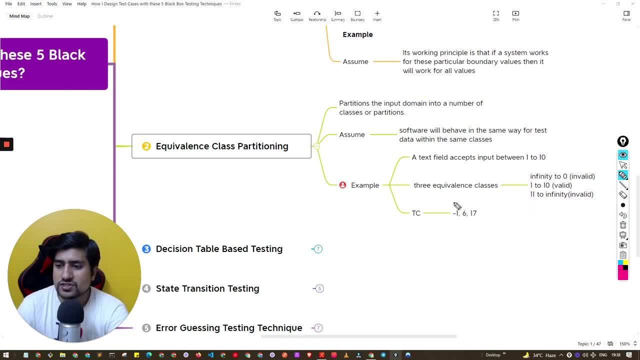 and this is your positive part, right? So here, if you see, I have just added three equivalents, which is minus one, in the negative part, in the positive part, in the positive part. So, positive, let me make it yellow. 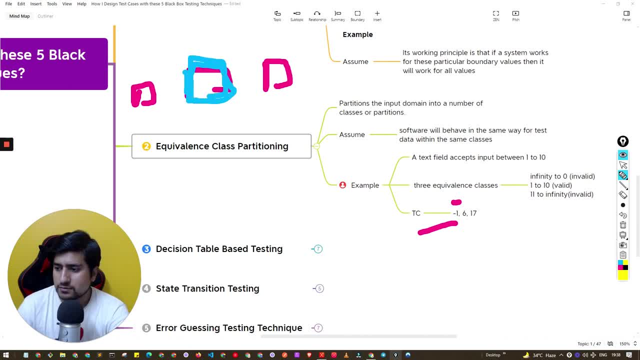 Ah, yellow, Okay, Click Okay. So this is yellow, So here. so this is one and 10, right, So here you can say: minus one is in your input six. you can take random any value between this six. 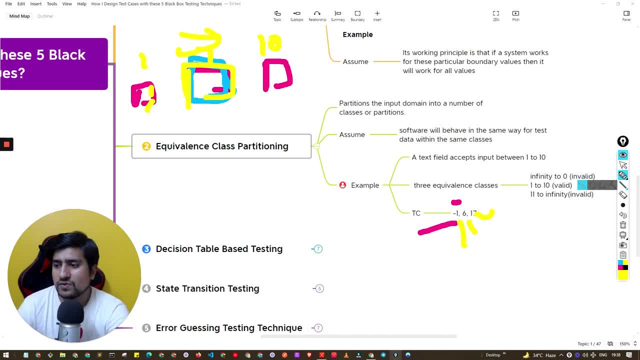 and the 17, outside the 10, above 10.. So this will be your equivalence partition for this. So now you have total number of cases: nine test cases, six with the boundary value and three with the equivalence partition. Clear, Clear, right? I hope this is very, very clear now. Okay, awesome. 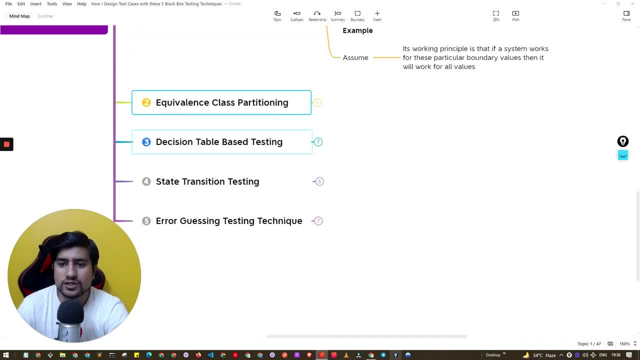 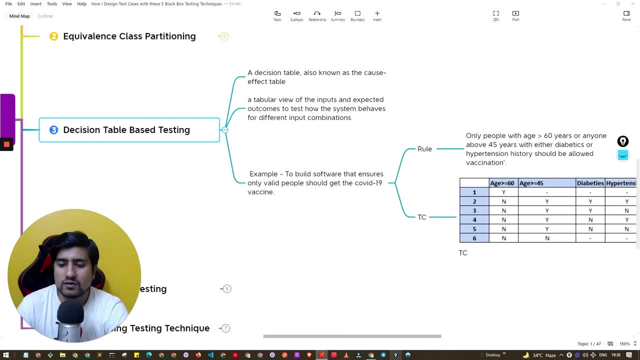 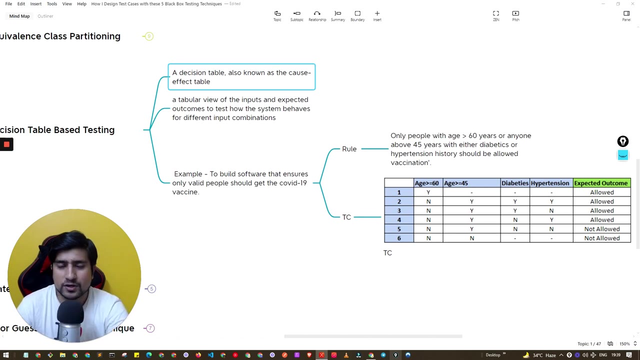 Please shut up. Yeah, Okay, Let's move on to the. let me close this also. Let's move on to the decision table. This is very simple, where what we are doing is basically a decision is created, a decision table is created to basically talk about the cause and effect of a particular test. 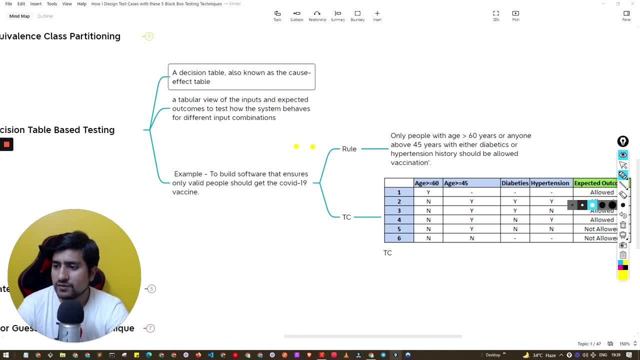 cases. So simple example. Again, we'll take a simple example. This is actually. there is a particular rule. For example, we have a table. we have some rule: okay to give the vaccination where we want to give vaccination. Okay, If the person is above 60. 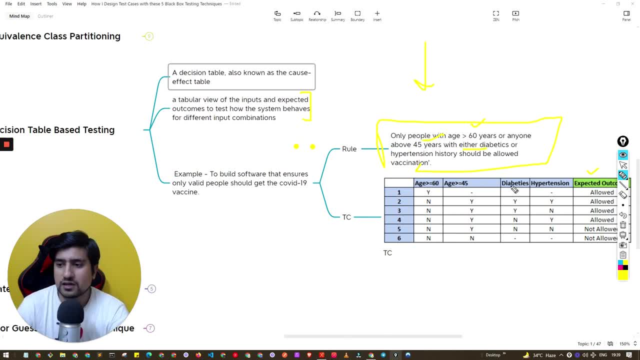 and less than this either have a diabetes or hypertension. Okay, So what we have done is basically we have created a yes or no kind of a table view. Okay, So if you see the row number, the row number one says the person is age 60. So there's no chances less than greater than 45,. 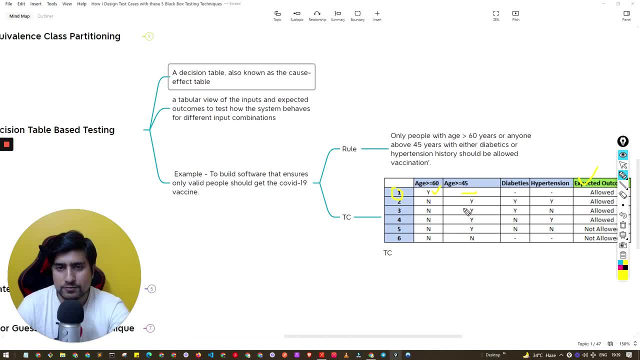 right, No diabetes. no, So the vaccination is allowed. suppose, Okay, And let's take this example where the person is basically greater than 45, but it is not. it is not 60 as of now And there is only hypertension. is he has only hypertension. There's no diabetes, So vaccine. 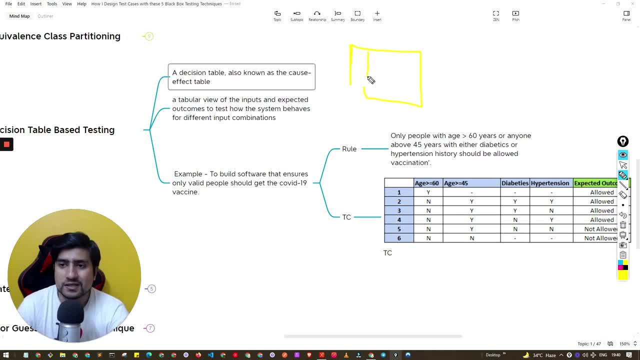 is allowed, right? So this is how, basically, what you are doing is. you are basically creating a tabular view of your decisions. What will the cause and what will will the effect on this? Okay, So to build a software to ensure that only people should get a COVID-19 vaccination. 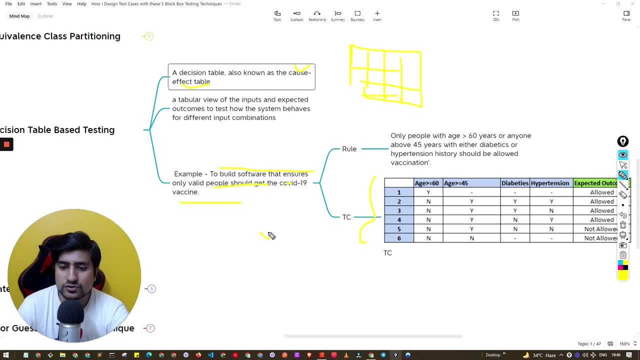 they have created this example. So these are your test cases now. So if you see, with a simple rule, with a yes or no, yes or no, that we have basically allowed and all right, We have created six test cases which will cover maximum combination and basically cover all the test cases related to this. 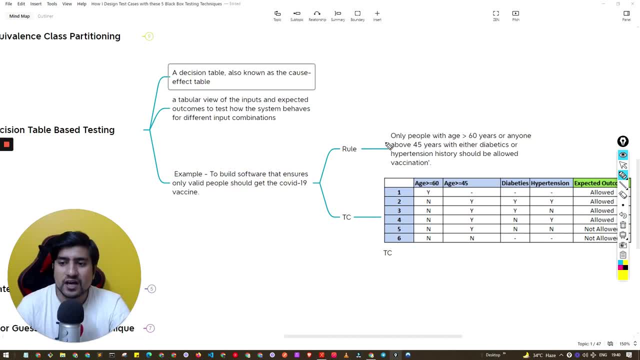 vaccine. I hope this is clear. Let me reiterate in a very simple way. There was a problem: who will get the COVID vaccine If we have a greater than 60 or greater than 45, if they have diabetes or not? So, based on that, they are allowed or not allowed to take vaccine. Okay, So those things we have. 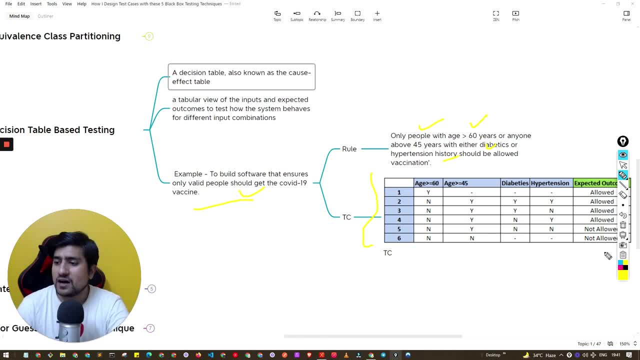 created in a tabular form. this is called as decision-based testing, And it's really easy And, trust me, it basically saves a lot. And you will- even- I mean with 10 years of experience- I'm telling you- you will face a multiple scenario where you have to create a decision table. I'm 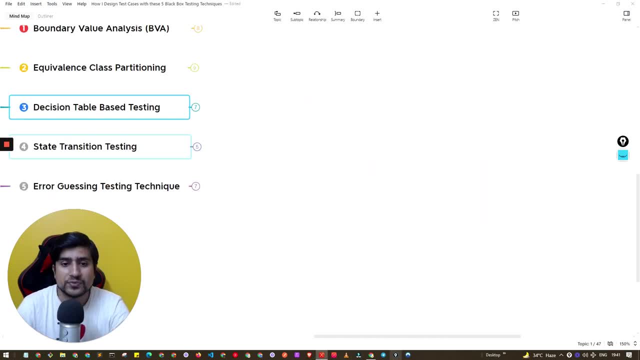 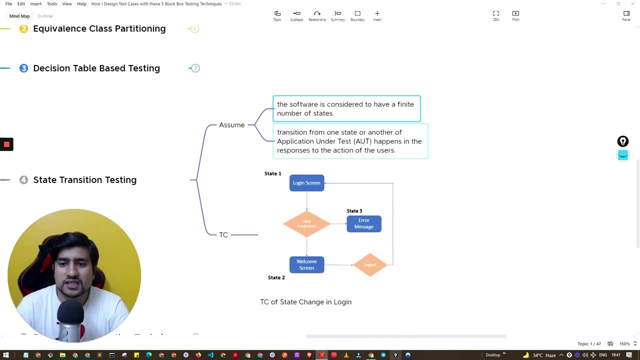 telling you to create your test cases. Trust me, Okay, State transition. Where, where are you? Okay State transition. basically, state it assumes, again, assumes, the software is considered to be have a finite number of states. So, for example, you are logging in, there will be a successful. 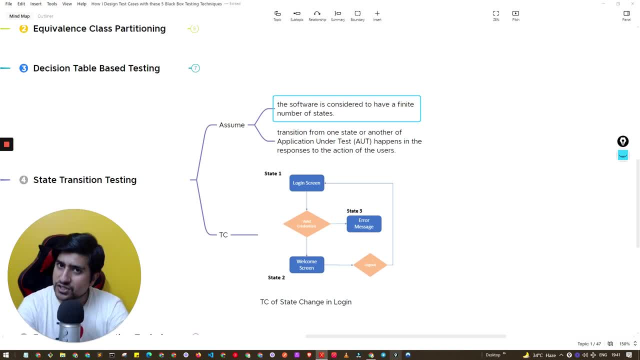 login. So that's a state. There will be unsuccessful login. There will be a state. So after successful log-in, there will have a dashboard page. this is your state. Okay, So that thing you are keeping in mind in here. All right, So we are assuming that there will be a finite number of states There? 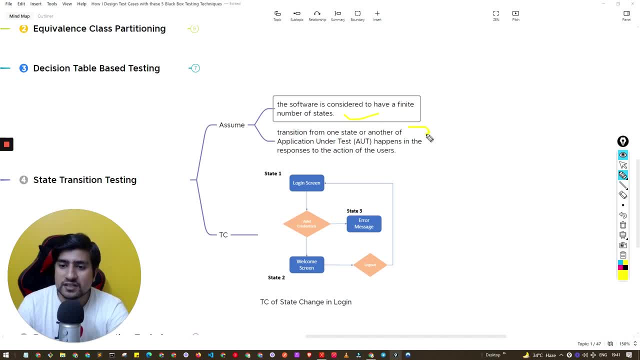 will not be infinite number of states in this case. Okay, And application under test, if you see, it will go from one state to another. that's it, This is what they are assuming. And now there, basically, I have taken some example from the online, where you have a login screen. 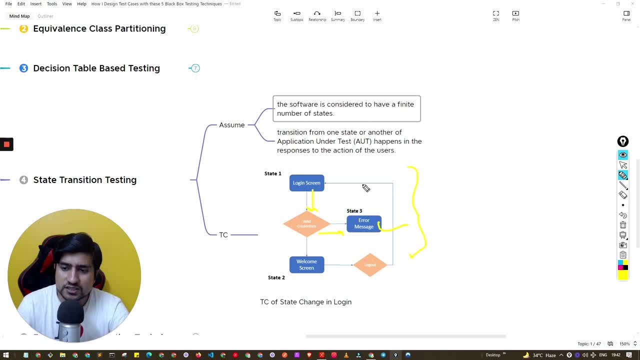 okay, After a valid login. if it is wrong, you will get an error message. This is your state. If it is valid, you will get a welcome screen and a logout button. So you have a screen you will see right. 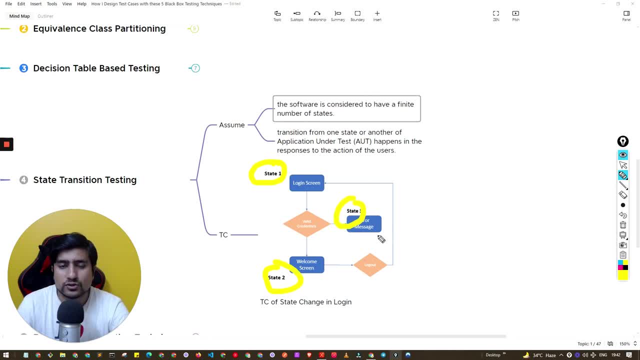 You have a state one, you have state two and you have state three. So you can say: based on this, you can create test cases- For example, valid credentials, invalid credentials- and there will be a logout button and you can create your number of test cases here. 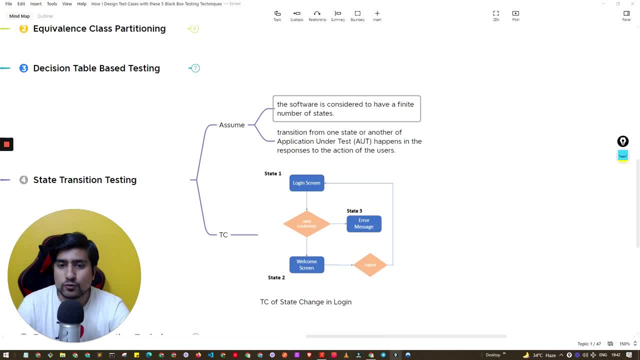 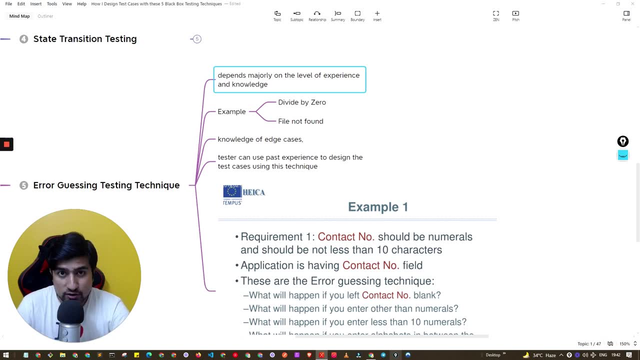 Clear, Based on the states, how your states are there for your software. That's it. Now comes to the error guessing, which is really, really important. It basically depends upon your level of experience. For example, divide by zero If there is a calculator-related app that you are testing. 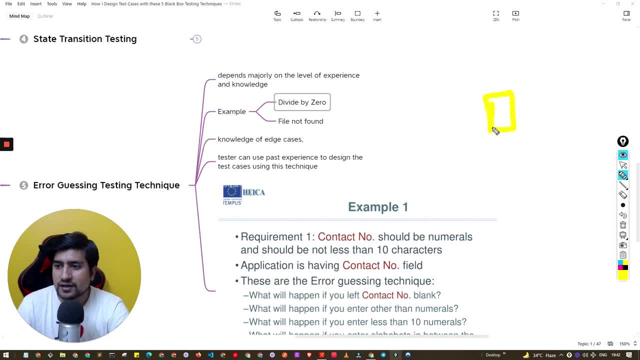 for example, you have a certain input field where people are entering zero by zero. then again, you know that it's a bug, so you will add test cases around it. So there will be one test case where you will add an input related to divide by zero. 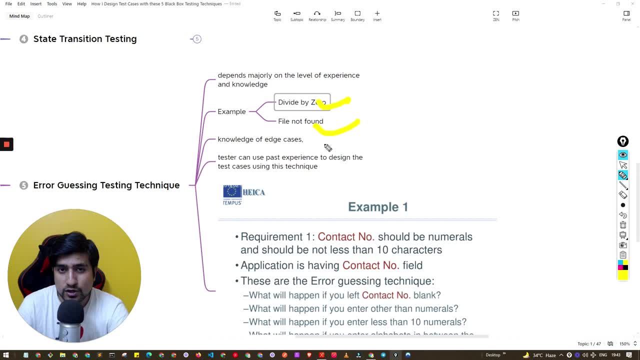 File not found. If there is a file-related test cases or a project that you are doing, then definitely you will add it right. So here you will see. it's a basically The edge cases we need to basically add in the error guessing. 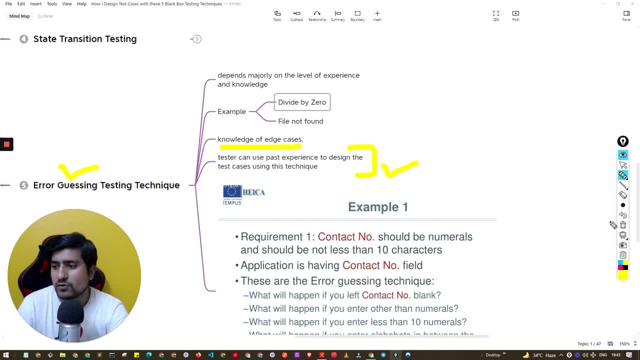 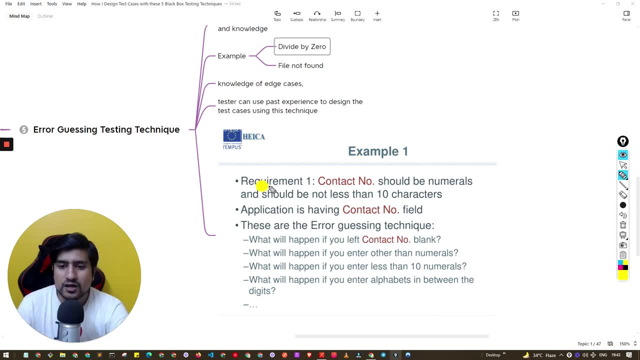 and testers can use a past experience and design your test cases around it. For example, if you see here right, They have added a couple of test cases based on the errors. For example, requirement is their contact number should be number, 10-digit number right. 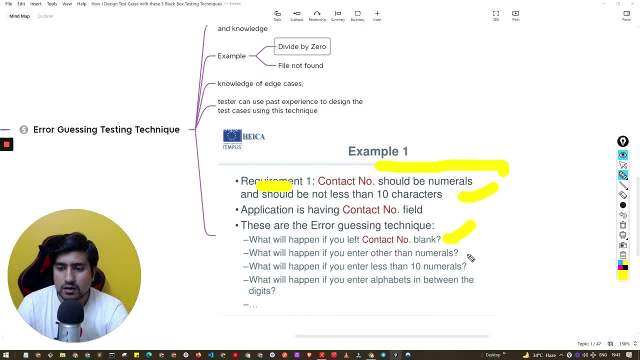 So what will happen if the contact is left blank? Other than numerical, they have added alphanumeric, They have less than 10, between 10, and there are multiple ones. So these are error guessing. They are guessing the What we call test cases and they are creating test cases around it. okay, 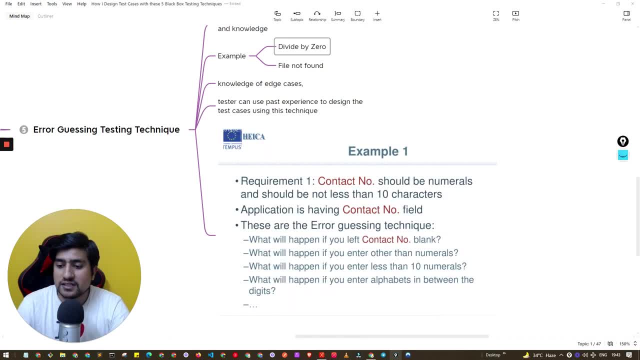 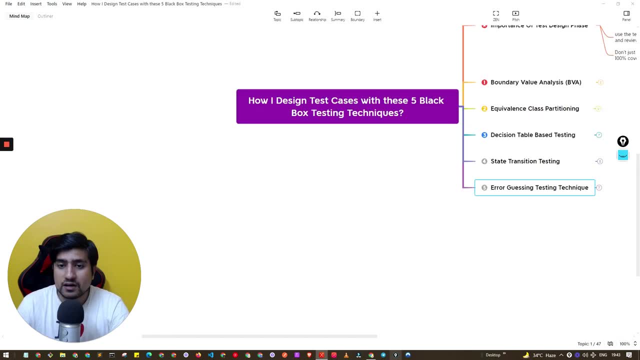 So those things- now I hope this is clear- guys Like these five techniques are really, really helpful to basically create the test cases. okay, I hope this is helpful And, trust me, this is the best example that I have prepared for you guys. 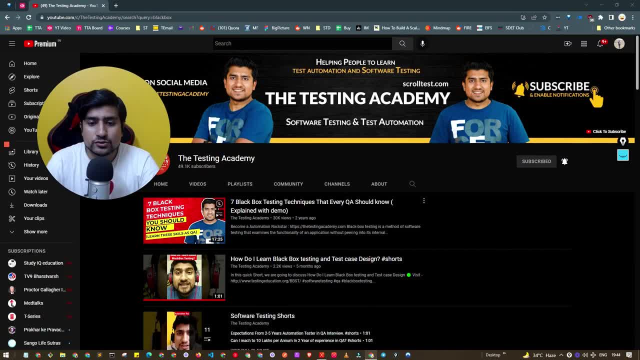 And, trust me, it will be helpful. One more thing I would request you. if you want to know more about two more techniques, you can watch the seven black box testing technique video. You can just go to the Testing Academy channel and go search for black box. 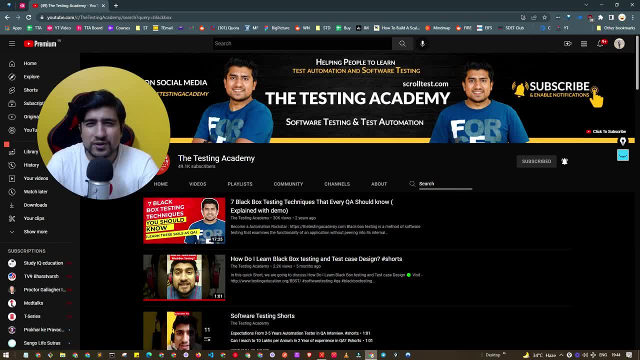 You will find this one. Please make sure you subscribe also. This will help me a lot. Near to 50k. please do that. all right, I'll see you in the next video. This is your host, Pramod.